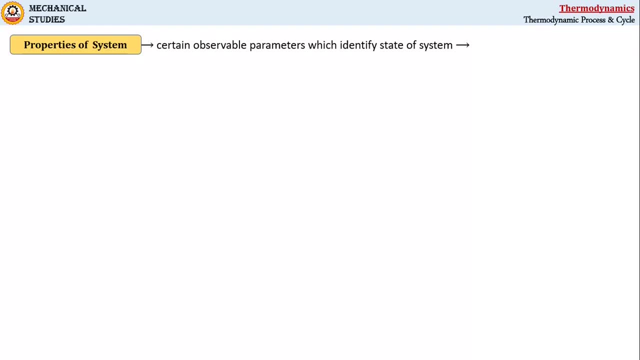 the bucket as a system, then the condition of the system that is water here, whether it is hot or cold, can be specified by its temperature. Thus all such parameters like mass pressure, volume, temperature, enthalpy, internal energy entropy and so on, 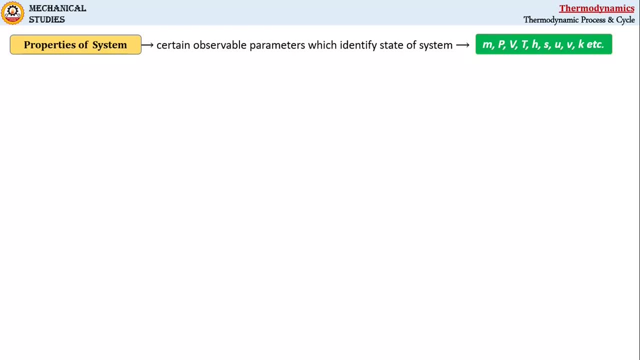 serve as properties of the system. Now these properties are of two types. First one is extensive properties which depend on the size or extent of the system, like total mass, total volume, total momentum, etc. And second one is intensive properties which are independent of the mass of the system. 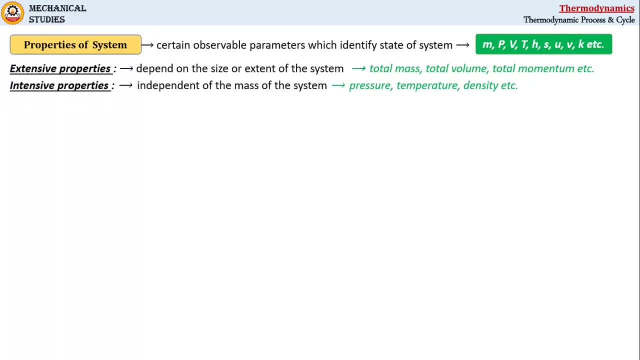 like pressure, temperature, density. And third one is specific properties, like specific enthalpy, specific entropy, etc. Now remember here: the ratio of any extensive property to mass of the system becomes average specific value and hence it is an intensive property. For example, specific volume is an. 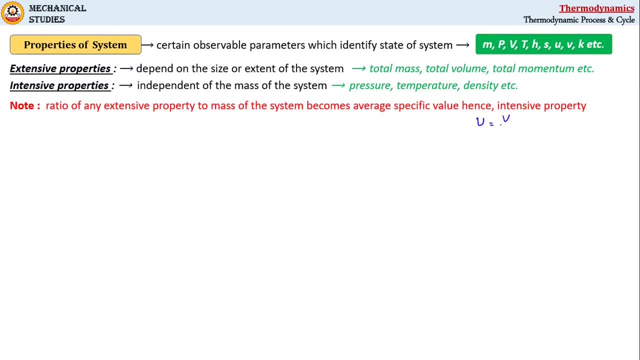 intensive property, which is the ratio of total volume to the mass of the system. or another example is specific entropy. So this is the ratio of total enthalpy to the mass of the system. Now, after discussing system properties, we will go to thermodynamic process. 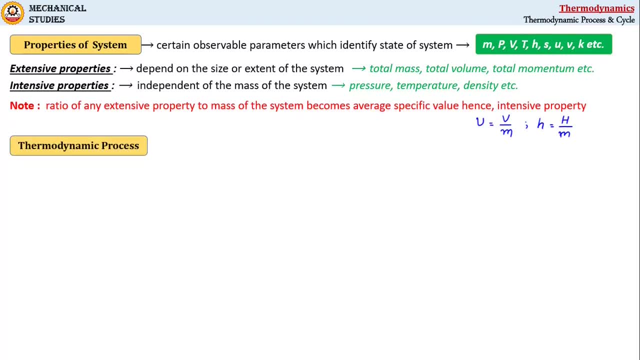 We know, a system undergoes a thermodynamic change. Thus, any change that a system undergoes from one equilibrium state to another is called a thermodynamic process, or simply a process. Now, in this study, we describe this change on property plots with the help of system. 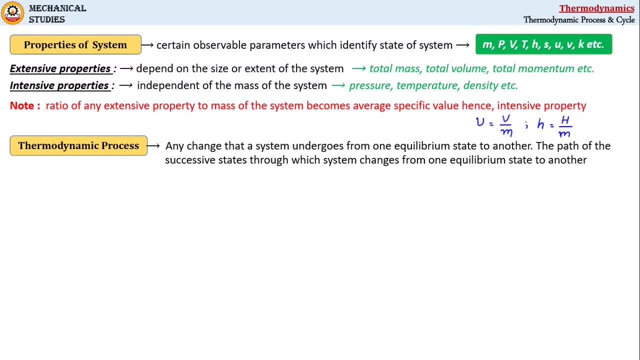 properties. Thus a process can be again defined as the path of successive states through which system changes from one equilibrium state to another. For example, let's consider here compression process of gas enclosed in piston cylinder device. Here A fixed mass of gas enclosed in cylinder is actually a system whose initial and final 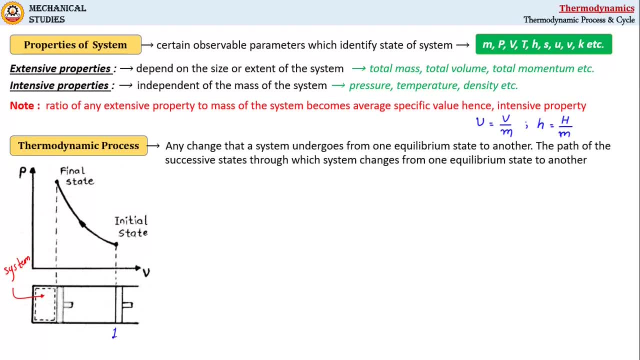 states are 1 and 2 and those can be represented, with the help of properties, pressure and volume on property plots as p1- v1.. Here it is p1- v1 and p2- v2.. Now let's consider a system: Pressure- p2 and volume- v2.. 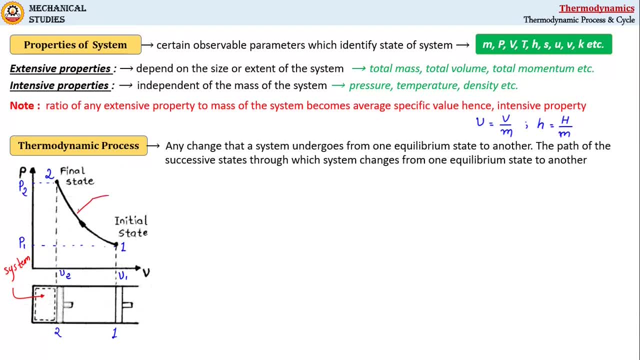 Thus, here, the path of successive states followed by a system during its change from one equilibrium state to another can be called as process. Now see, all actual processes are very difficult to analyze since in this case, only initial and final state are at equilibrium. Therefore, these actual processes are modeled and analyzed as Cauchy static process. 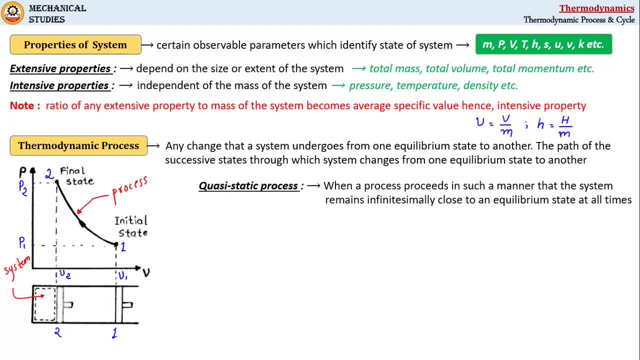 A Cauchy static process, or also called as Cauchy equilibrium process, is the process in which all intermediate states remains infinitesimally close to an equilibrium. So don't forget here- important point- that Cauchy static process is not true representation of actual process, whereas it is an idealized process which is being a standard to which 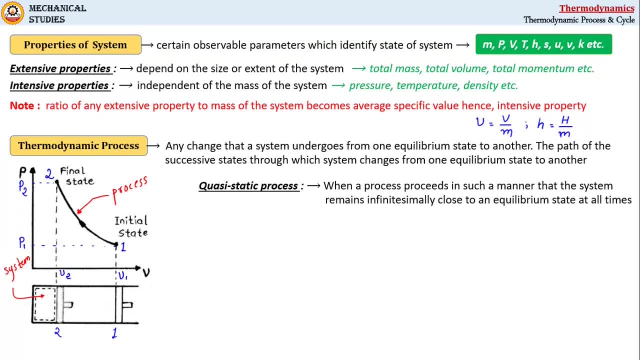 an actual process is compared. This is being done because of two reasons. First one is Cauchy static process is easy to analyze and second is work producing device deliver most of the work when operated in Cauchy static manner. For a process to be Cauchy static. 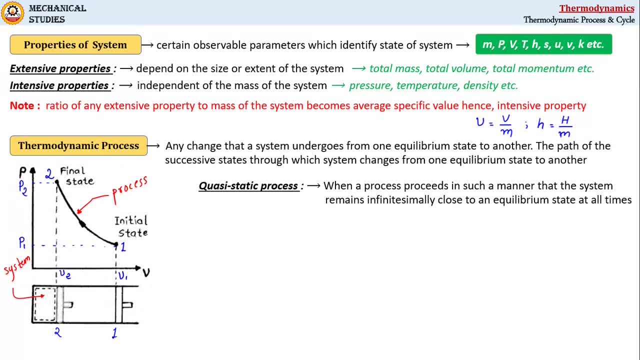 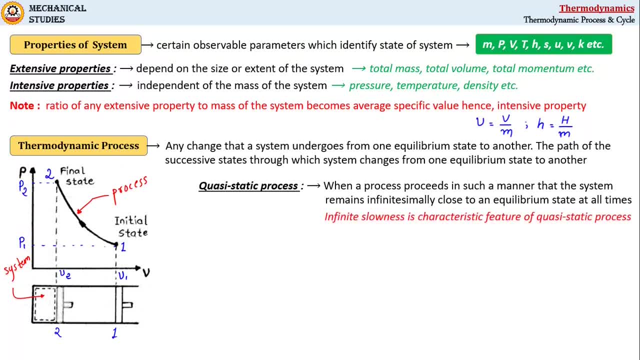 It has to be carried out very slowly. that means infinite. slowness is a characteristic feature of Cauchy static process. Now, one important term is here that we must not skip, which is reversible process. Reversible process is the process through which system can be restored back to the initial. 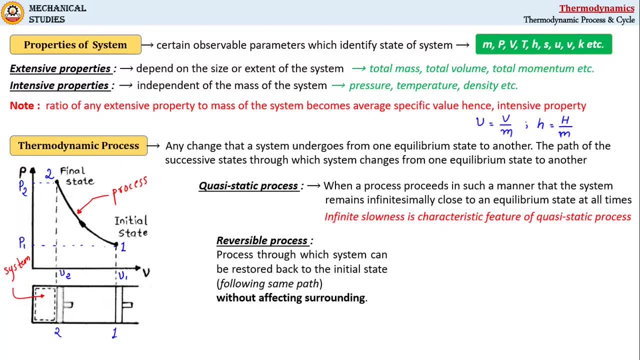 state following the same path without affecting the surroundings, Without affecting the surrounding, Without affecting surrounding. These are very important words from this definition. Without these words, the definition of reversible process has no sense. Reversible process is impossible to achieve in reality and I will tell you why. with a 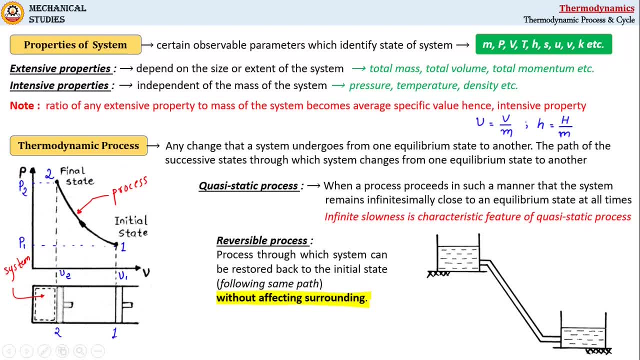 simple example here Let's consider water flowing through pipe connected to two tanks, Tank A and Tank B, Separated by elevation difference here. So here water will easily and by default flow from tank A to tank B because of elevation difference, which is a natural process. 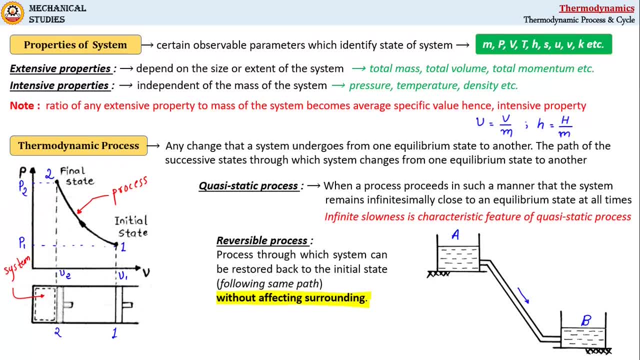 Now the question comes: can we make this process reverse? One can say, definitely, we can do this task with the help of pump here that lifts the water from tank B to tank A through separate pipes, Through same pipe. So can we say this reversible process? 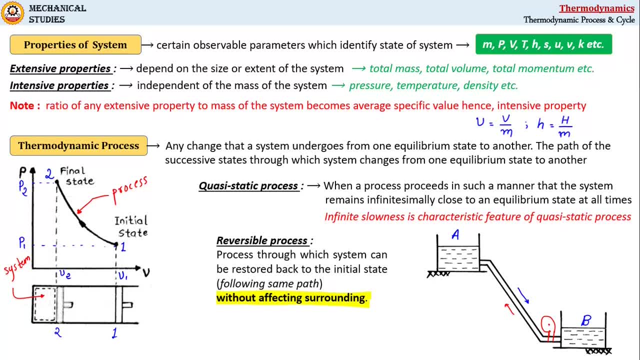 The answer is no. We cannot say this reversible process, and I will tell you why. If we look at the system here, the system comprises of tank A, tank B and the pipe connected between these two tanks. Anything outside of this system will be surrounding here. 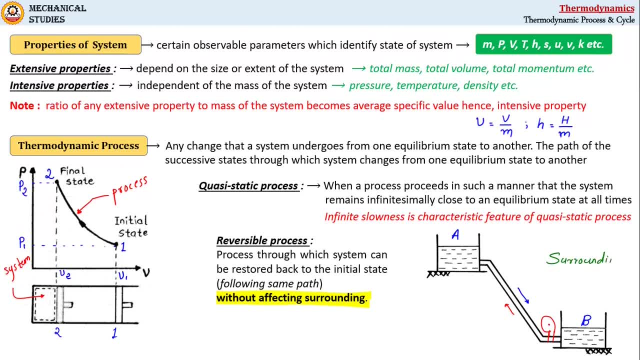 Okay, And in order to perform the task to this pump, we must supply energy to this pump from outside, obviously, from the surrounding, And this is why the surrounding is getting disturbed here. Okay, And that's why, as per the definition, we cannot say this as a reversible process. 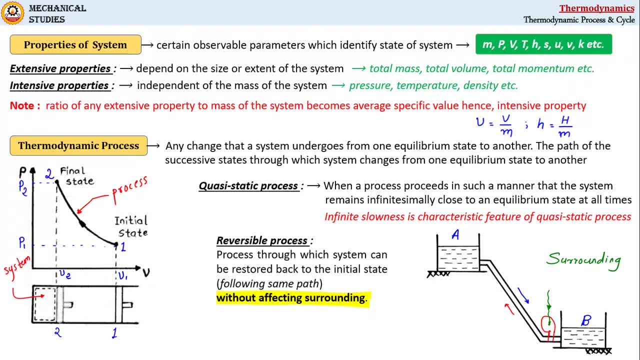 It's a irreversible process. In fact, all the processes are irreversible in nature. Various factors causing the process to be irreversible are called irreversibility, And these factors are like elevation difference, potential difference, finite temperature difference, magnetic hysteresis, fluid friction, static friction, etc. etc. 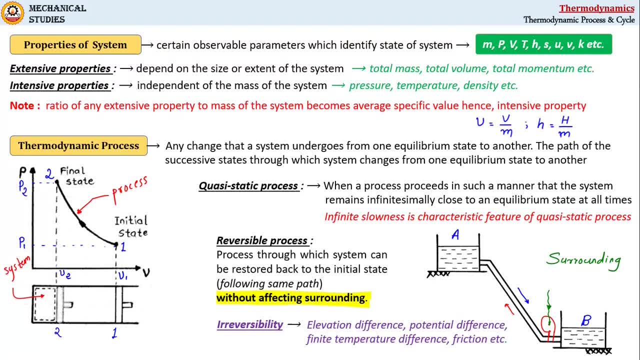 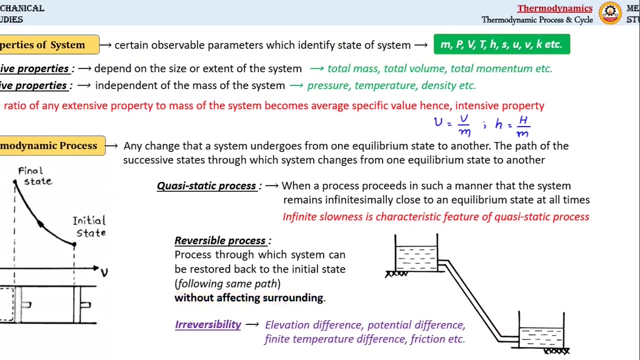 Okay, Now these irreversibilities are always present there in a system and we cannot completely remove these irreversibilities from the system. Okay, All the processes are irreversible in nature. It is very difficult, rather impossible, to create a reversible process. We will go now to the next term, that is, thermodynamic cycle. 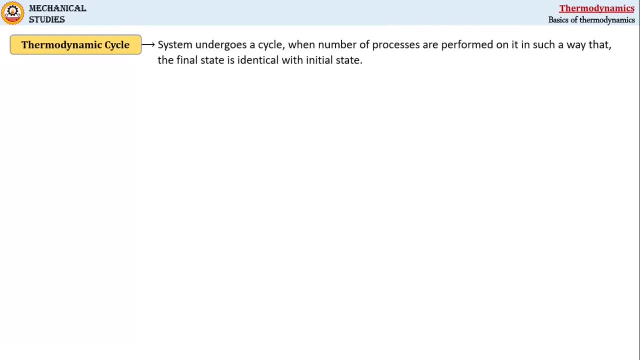 And we can say: a system undergoes a cycle when number of processes are performed on it in such a way that the final state is identical with initial state. Thus The cycle system is restored to its initial condition. For example, here the system undergoes a thermodynamic cycle with two processes, with 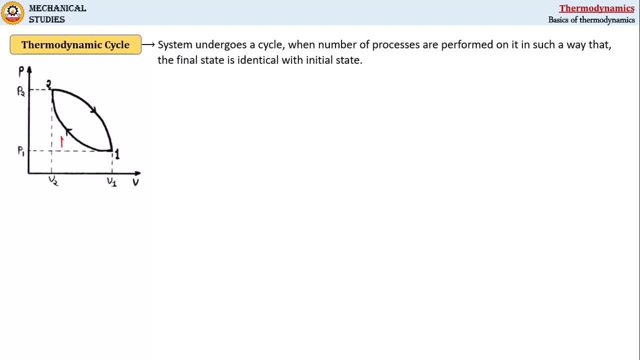 different paths, Let us say path A and path B. Thus the two processes those are comprising cycle here will be represented as 1A and 1B. Okay, This is our cycle, And second process, from 2 to 1 through B, that will be represented as 2B1. 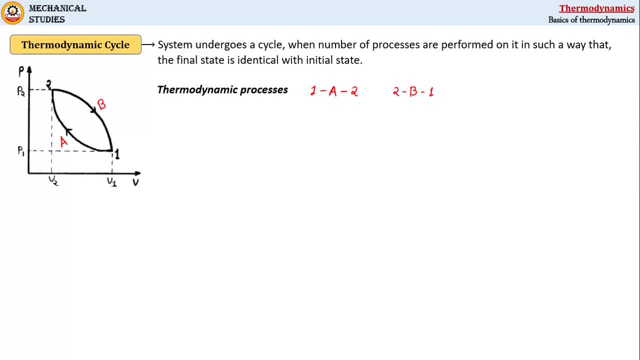 Okay, whereas the entire cycle can be represented as 1A2B1.. So you can see, here the system comes back to its initial condition, that is, 1.. This is the initial condition I am talking about. This is the initial condition. 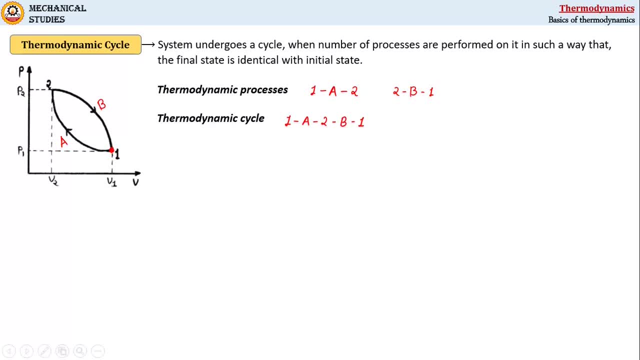 First, In this subject you will come across various thermodynamic cycles and their corresponding property plots. That's why it is very much essential to understand the properties and their application in describing process as well as cycle. I will summarize this discussion here with an example of diesel cycle, where we can see 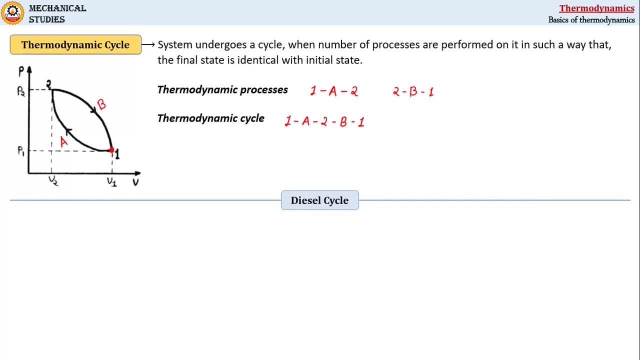 how the properties are used to describe processes and cycle. These are pressure, volume and temperature entropy plots of diesel cycle that consist of four processes. First process 1 to 2, that is isentropic compression of air. Second, process 2 to 3, that is constant pressure, heat addition.